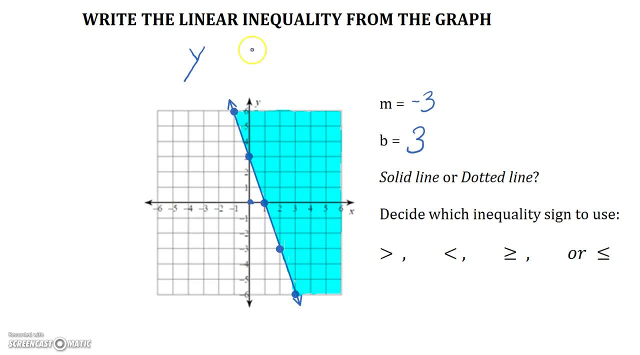 y Something negative, 3x plus 3.. Our next step is to identify the type of line. Looking at the line, it is solid. So right from the get-go we can eliminate the greater than and less than sign. 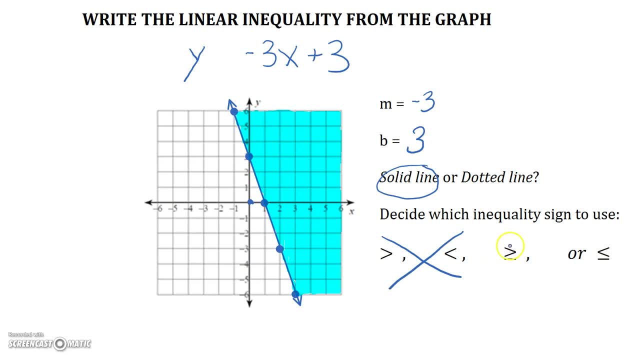 Because solid lines are either greater than or equal to, or less than or equal to. Now, just like in our previous video, we can use the point 0, 0 as a test point. So, taking what we already have of our inequality, we can actually plug that point 0, 0 in. 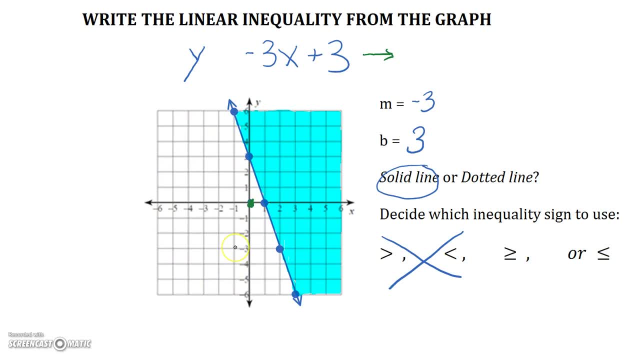 Now, if you notice, 0, 0 is not a solution to our inequality, because it's not part of the shaded region. Therefore, we're looking for a function, We're looking for a false statement, because 0, 0 is not included. 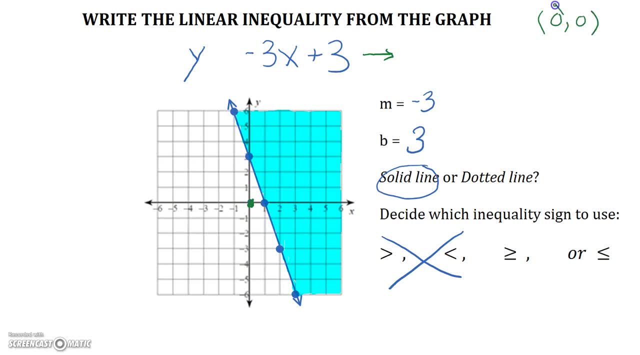 Let's try it. Okay. so we're plugging in 0 for y and 0 for x, So we have 0, blank negative 3 times 0, plus 3.. 0, blank negative 3 times 0, 0, 3.. 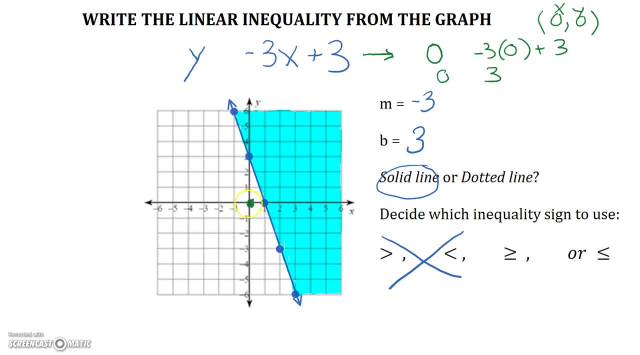 Now again, 0, 0 is not a solution to our inequality. Therefore, we want a false statement between the greater than and or equal to, or less than or equal to. We're going to use greater than or equal to, because this is a false statement. 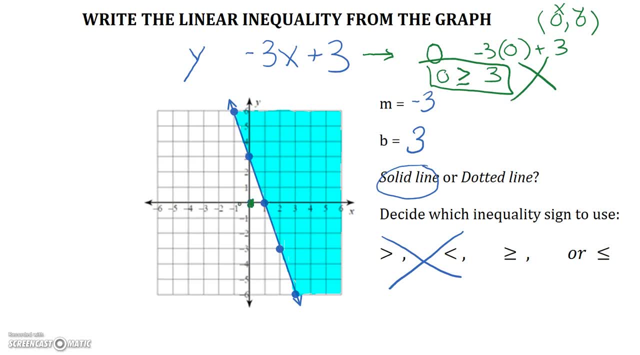 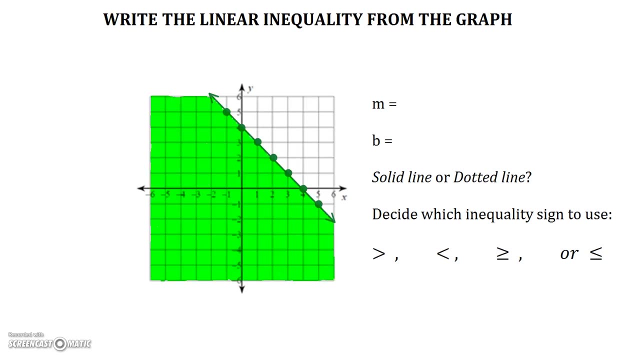 And we don't want 0, 0 to work because it's not shaded. Therefore, we're using greater than or equal to, and we're done. Let's try it. Let's say that we have less than or equal to, and we're doing 0 to 0, 0, 0 to. 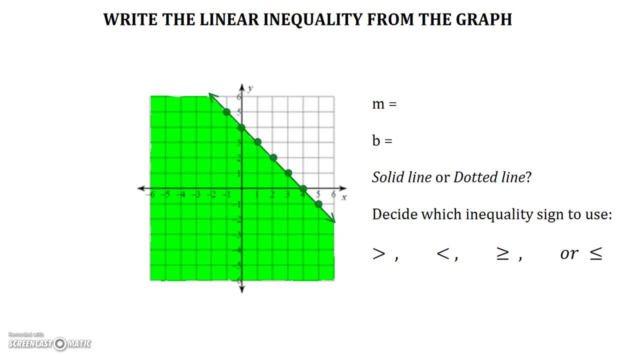 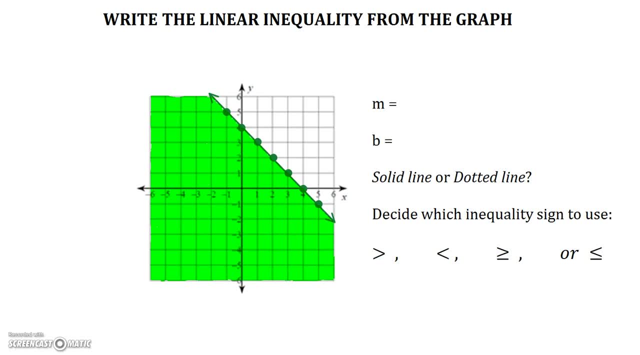